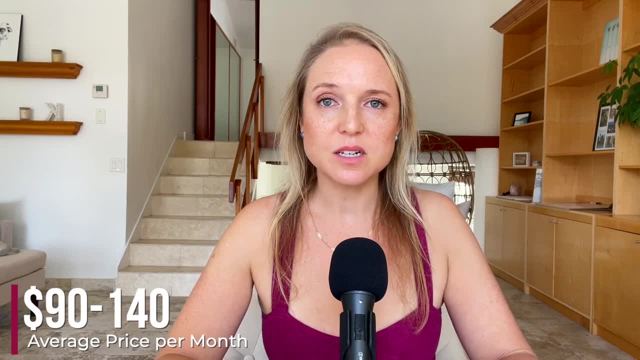 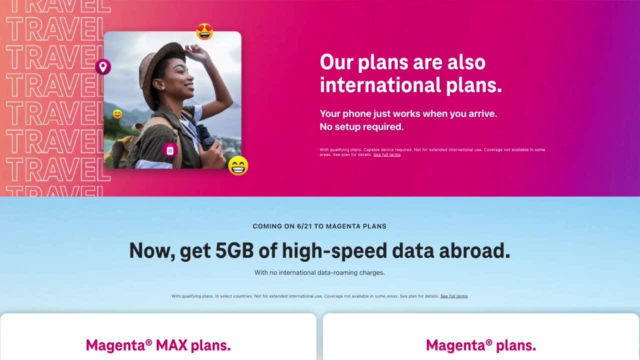 past is this T-Mobile international plan. They have one called the Magenta plan and this is good in also around 200 countries. The good thing about this is that you don't have to do anything. You just turn your phone on when the plane lands and you can immediately connect to the local. 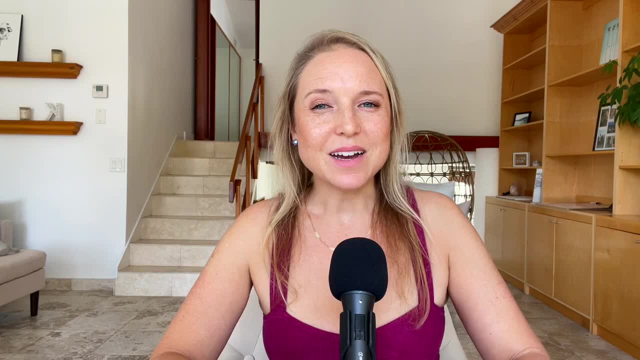 network, start texting, start talking to your friends and then you're good to go. So if you're using maps, the downside is that the speeds are really slow. We're not talking 4G or 5G here, We're. 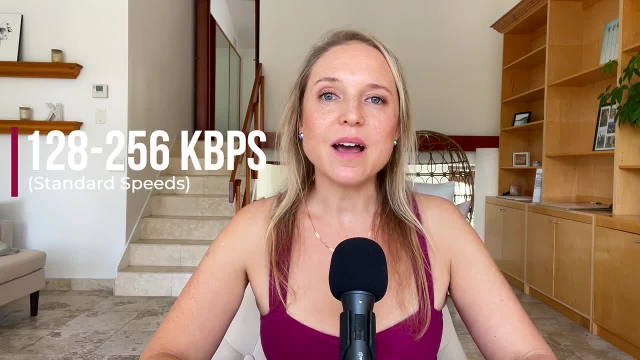 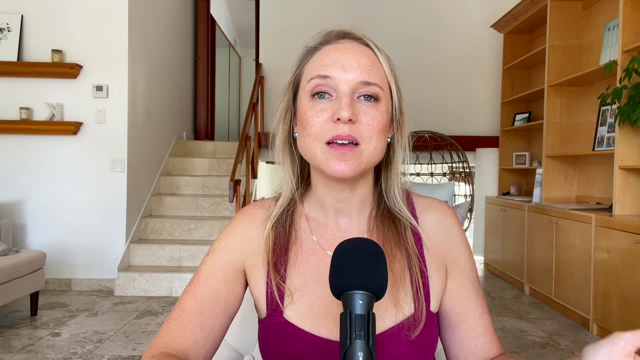 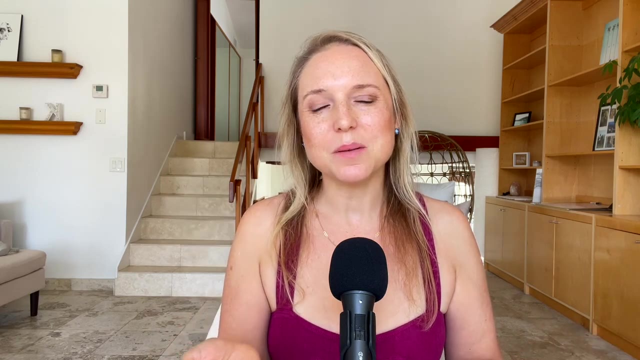 talking 128 kilobits per second. So I like to have two phones. I have my normal phone with the T-Mobile plan and I also have a separate unlocked phone that I can use with international SIM cards. So I like to have that T-Mobile plan because I can use it anywhere and it's good enough to send messages. 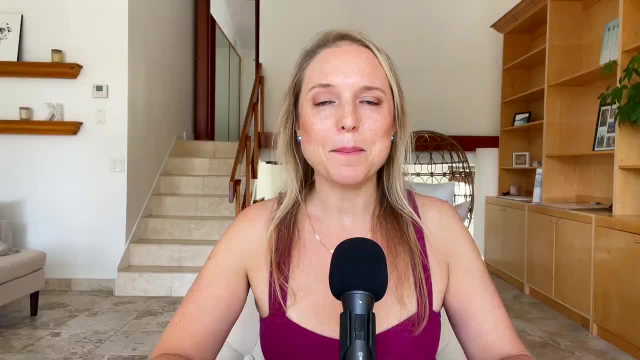 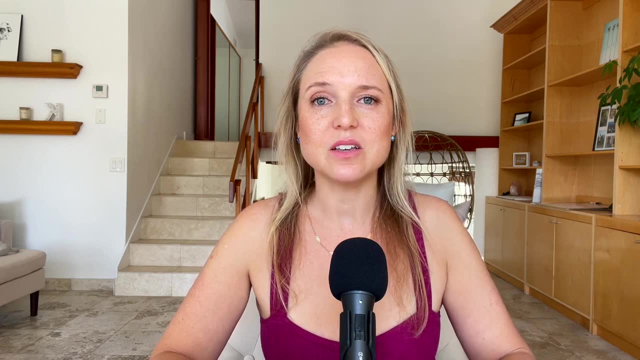 on like a messaging app or to use maps or something like that, But you're not going to want to be downloading stuff or streaming any kind of music or video. You really can't with speeds that are that slow And it can also get expensive too if you want to upgrade to a faster data plan. 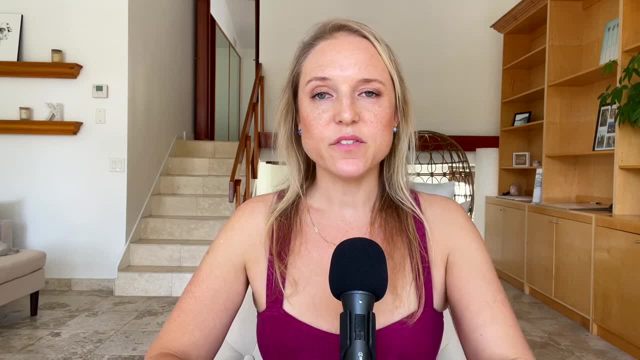 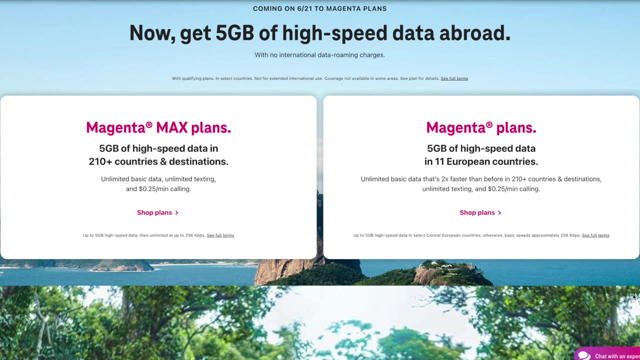 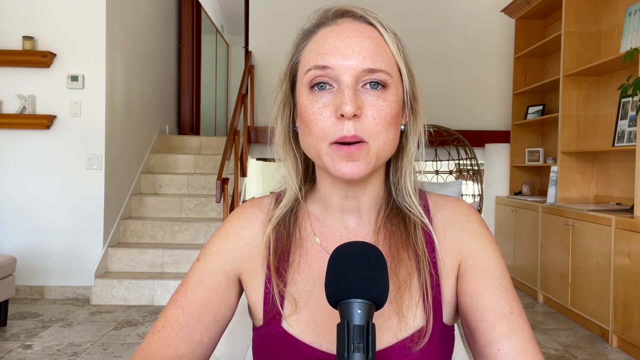 and it's still not even that fast. Consider this: If you were to upgrade to the T-Mobile high speed data package, you could get five gigs of LTE data for thirty five dollars, And only good for 10 days. So you need to triple that to have a high speed data for a month, and it's 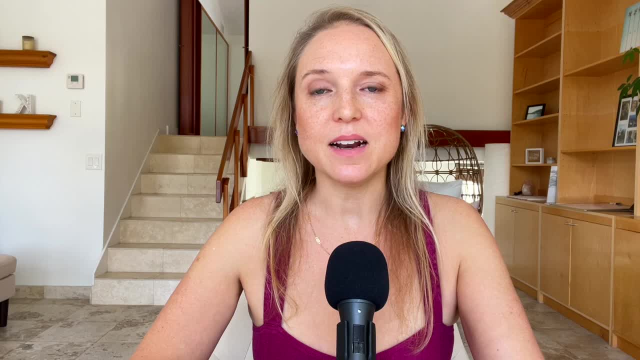 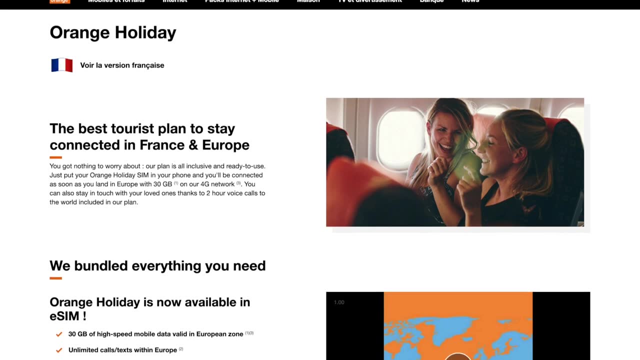 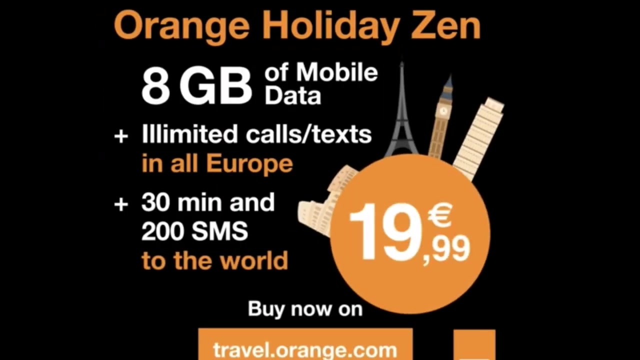 only giving you 15 gigs of high speed data. In comparison, if you bought a prepaid tourist SIM card in France, for example, you could get up to 30 gigs of high speed data for 30 euro, and that's good for 14 or 15 days. So that would be 60 euro max paying for high speed data. there You'd get. 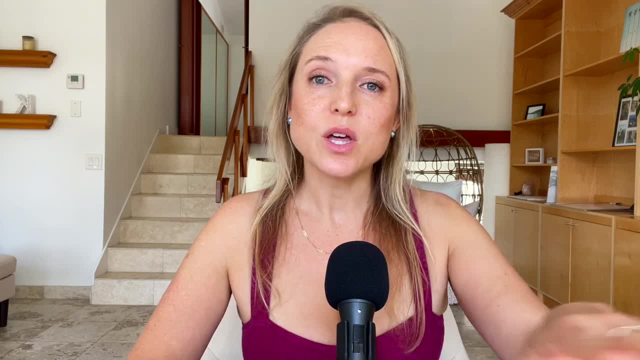 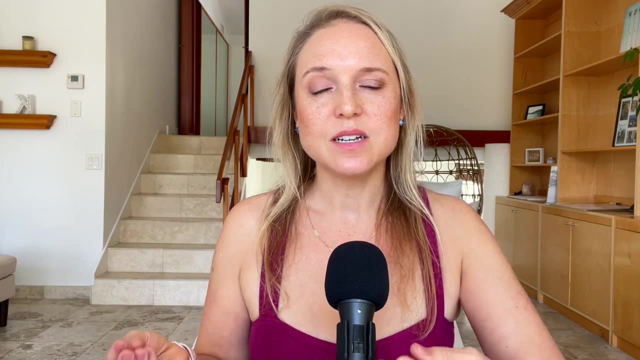 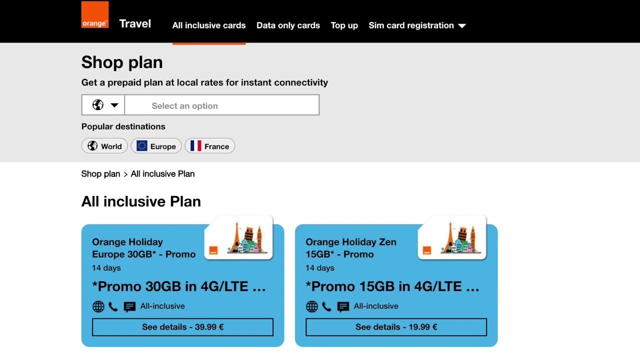 60 gigs of data, and that would also cover you throughout the European Union. So you can see how it's much more expensive to add an international data plan to your US phone compared to if you are going to buy a prepaid SIM card when you get to your destination. If you were to buy a prepaid 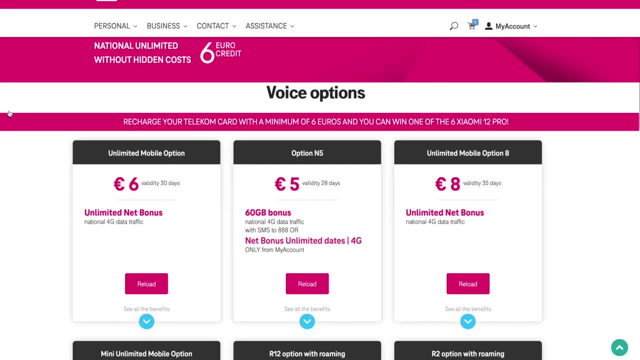 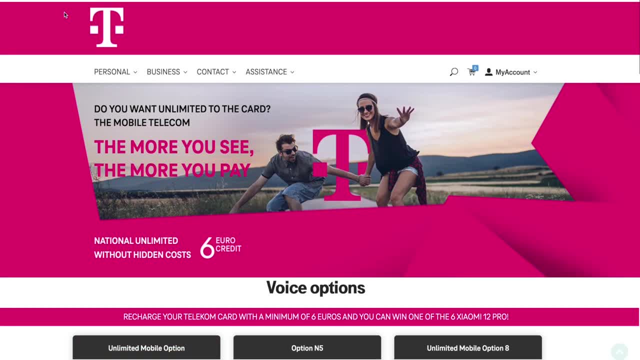 SIM card in Romania, you could get six gigs of data that's good for an entire month- for just six euro. Now if you're from the US and you're looking AT&T or T-Mobile, it is more affordable to go with something like Google Fi that charges you. 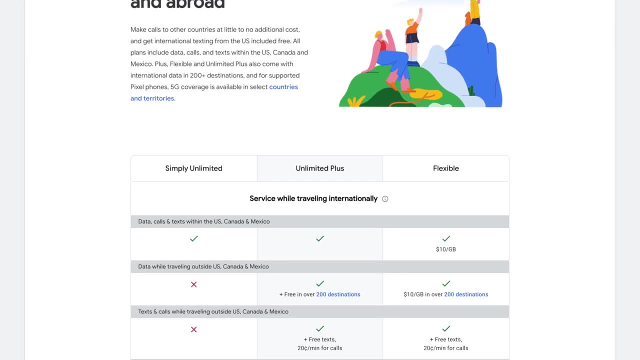 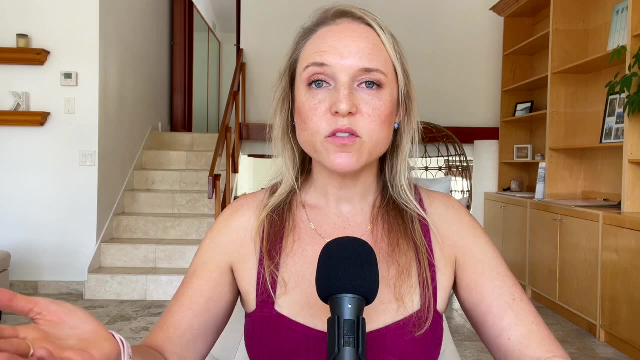 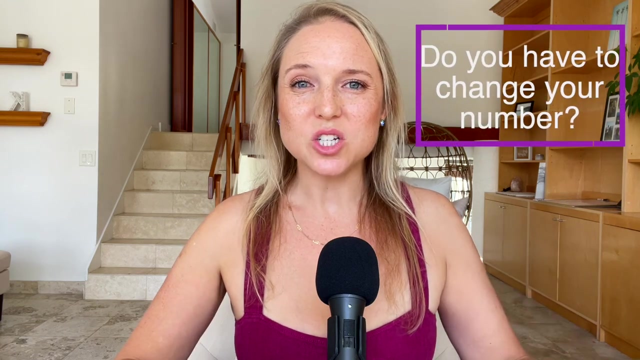 $10 per gig of high speed data when you're abroad, but that's still a lot more than paying for local data in the country where you land. So one of my clients asked me: well, what does that mean? if you're buying a prepaid SIM card in every country, Does that mean that you have to change? your number in each country that you go to. These days, there's a lot of other options. You can keep an international cell phone plan with a basic minimum data package with Google Fi or something like that, or you can also have an online number that forwards to different phone. 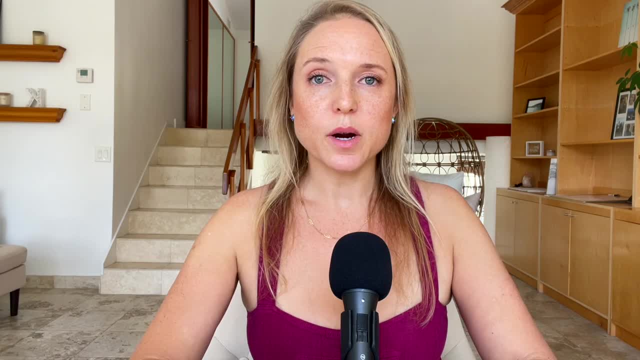 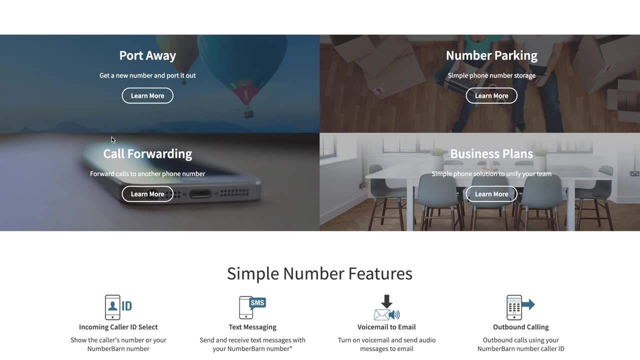 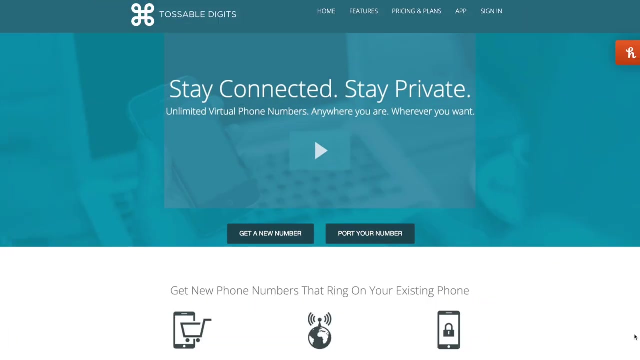 numbers that you have, So you can use Number Barn, Skype, Google, any website or online provider that lets you use a mobile number that you can answer through the internet or that can forward to your end result cell phone. One subscriber told me about a website called Tossable Digits where you can forward your phone number. 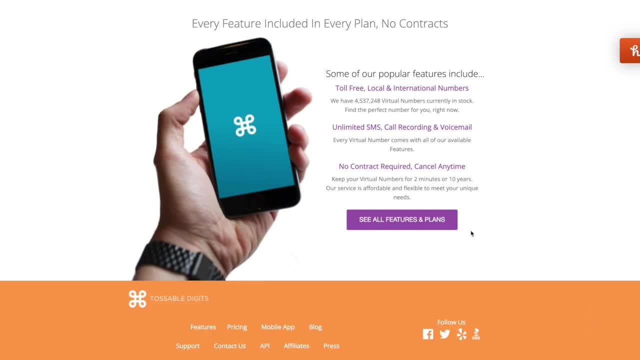 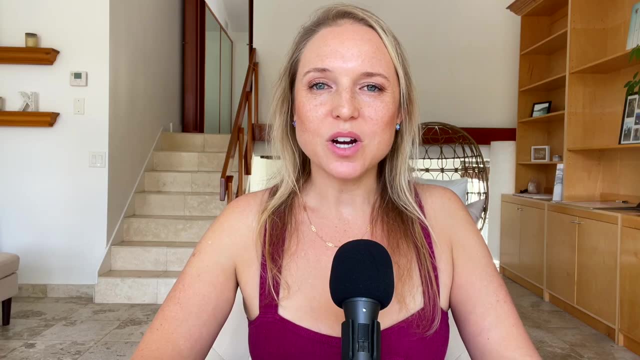 anywhere and receive text messages around the world. It also includes features like voicemail, call recordings and caller ID, So when you're thinking about traveling to multiple countries, don't worry about having to change your number wherever you go, because chances are you're going. 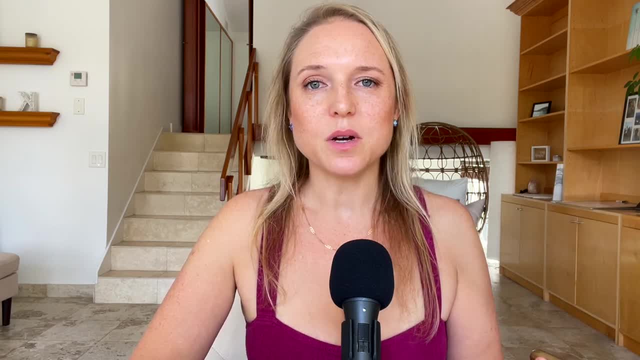 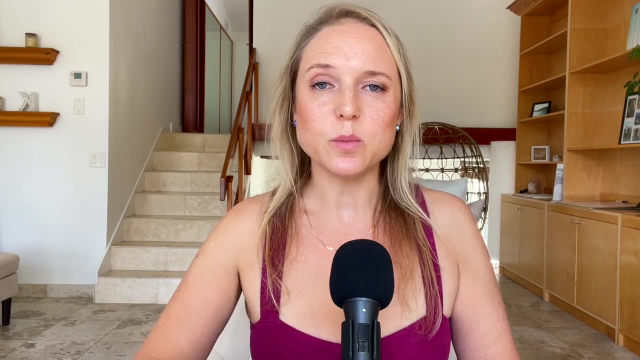 to be using your unlocked phone with a local SIM card pretty much just to use the internet, And if you need a internet connection you can just use the internet. If you have a phone that's not connected to your phone at all, then you can just email your authorized number or name. I think I already gave that up late. But if you have an international number or a US number for your business, then you can have that number forwarded to your international phone or you can just answer those calls online. However, if you don't add an international roaming plan to your home country phone, then make sure to. 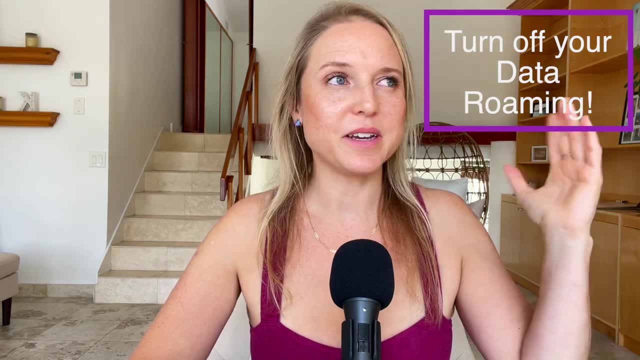 turn off the data roaming, because you can get a pretty bad surprise when you get home and check out your phone bill and you're getting charged like $100 per Gigabyte of data or something like that. So go into your phone's ass and then just fill out the information. settings. turn off your international roaming data if you don't have a plan specifically that lets you use your phone in other countries. but that's also an option as well, because there's wi-fi pretty freely available these days. sometimes there's public networks that are provided by the. 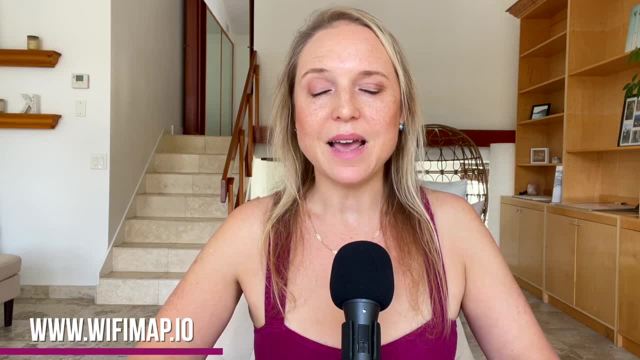 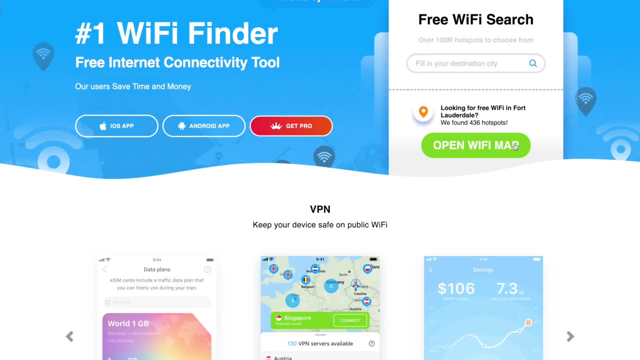 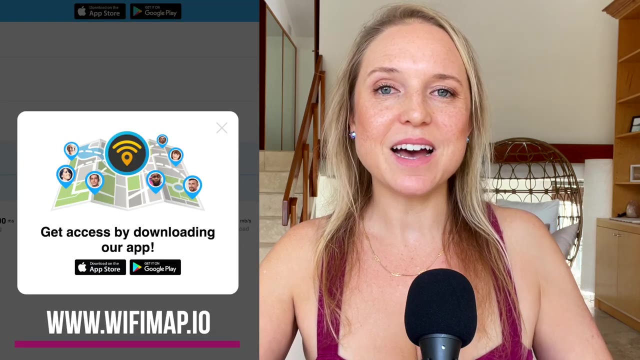 local government or municipality, and you can also download an app like a wi-fi map app or a wi-fi finder app that shows you where all of the networks are around you. so it's possible that you could even travel with just using the wi-fi wherever you go. but i like to have an internet.